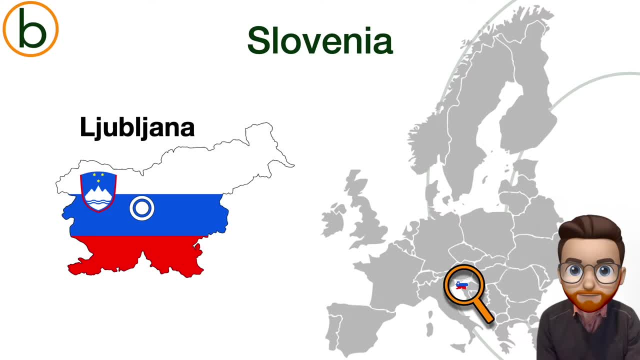 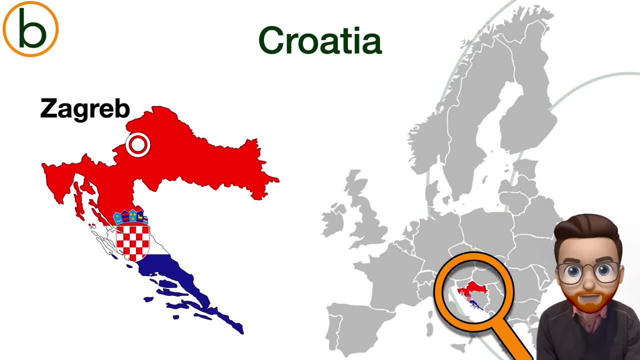 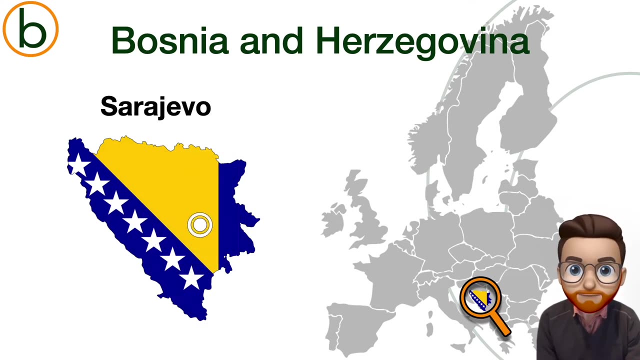 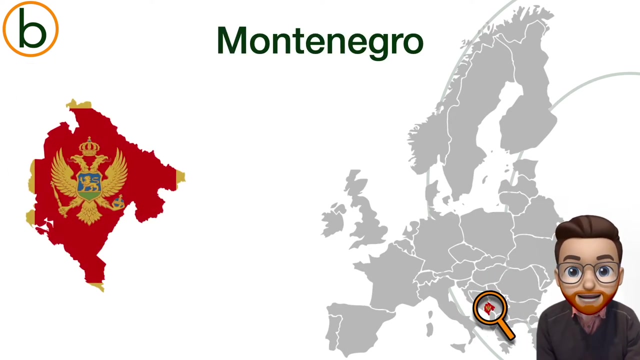 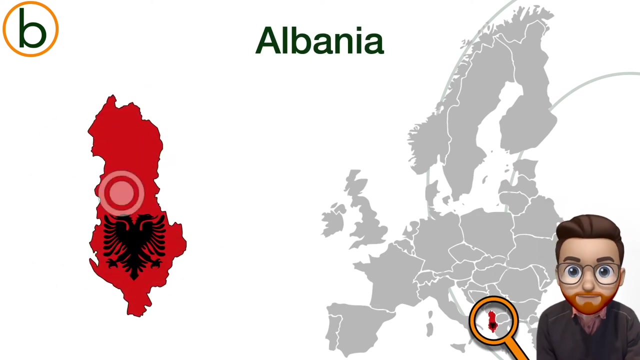 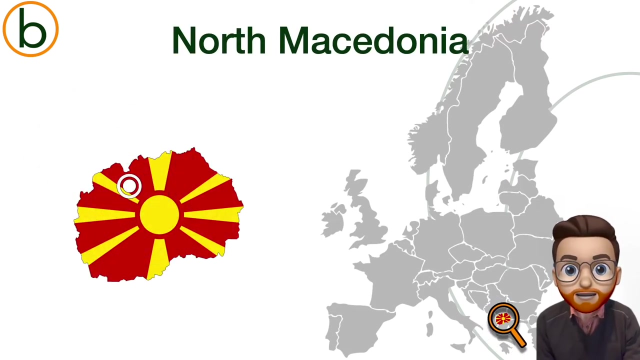 Slovenia has Ljubljana as capital. The capital of Croatia is Zagreb. Bosnia and Herzegovina has Sarajevo. Serbia has Belgrade. Montenegro has Podgorica as capital. The capital of Albania is Tirana. The capital of North Macedonia is Skopje. 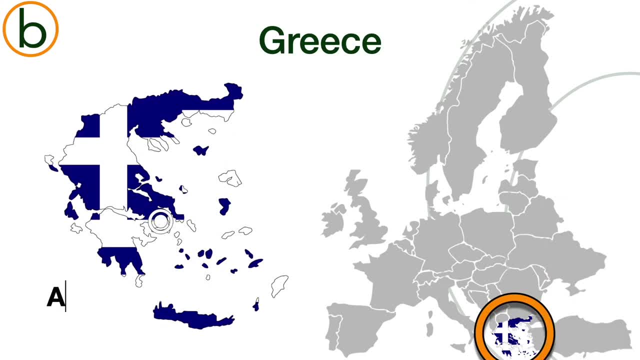 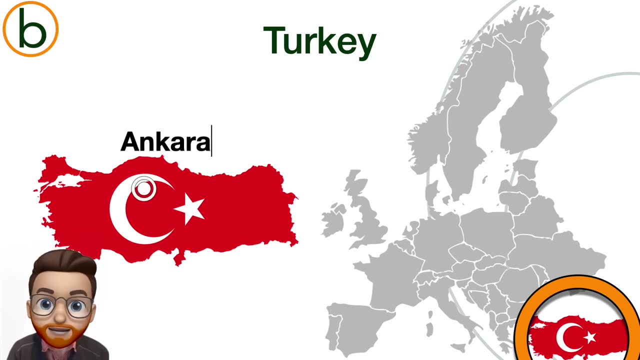 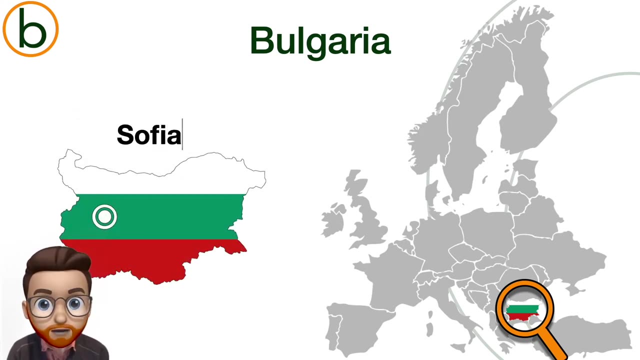 The capital of Greece is Athens. Bukovara has Eastern Europe. The capital of Poland is in the middle of the world. The capital of Hungary is Germany. The capital of Poland is Hungary. The capital of Lithuania, Austria, has the capital of Budapest. 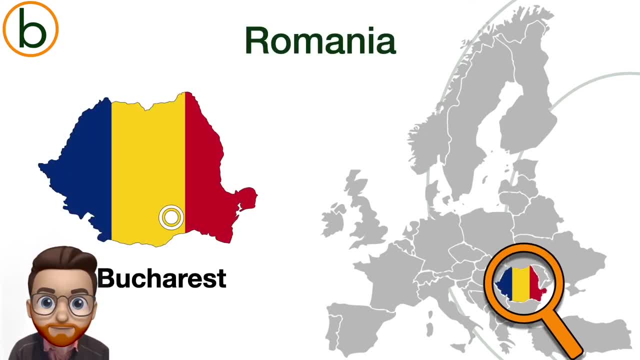 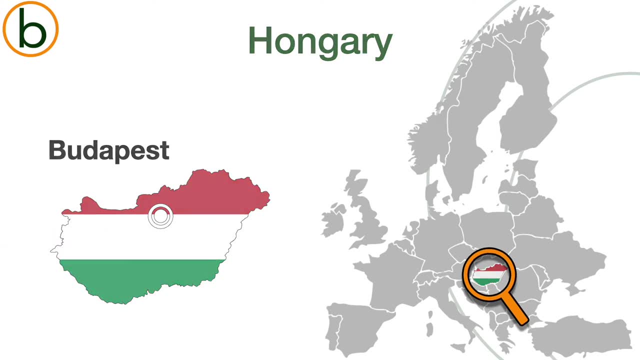 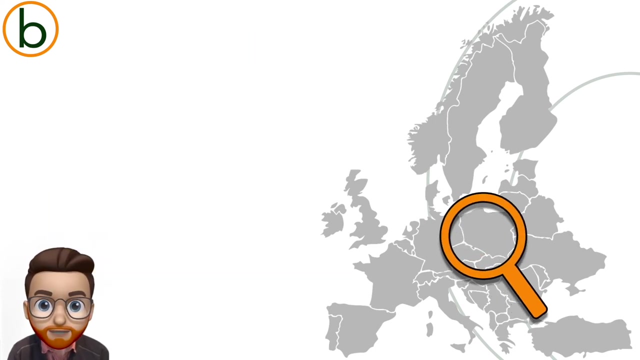 The capital of Spain has the capital of Germany. The capital of Hungary has Bohemia. The capital of Serbia has Stockholm. The capital of Hungary has Bolivia. The capital of Bulgaria has Turkey. Latvia has the capital, Bratislava. The Czech Republic has Prague. 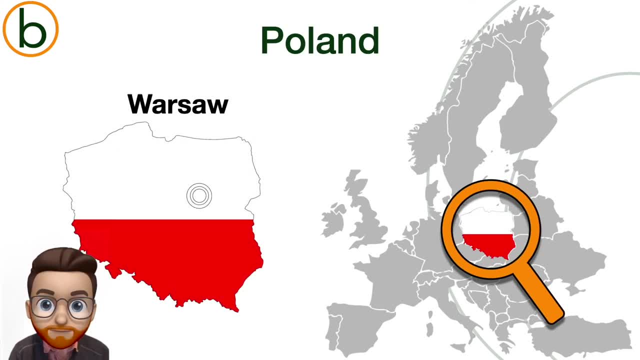 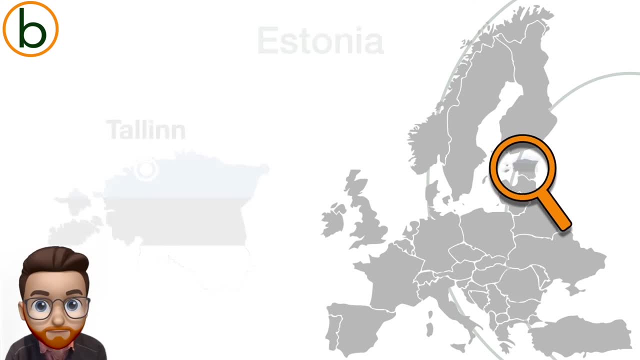 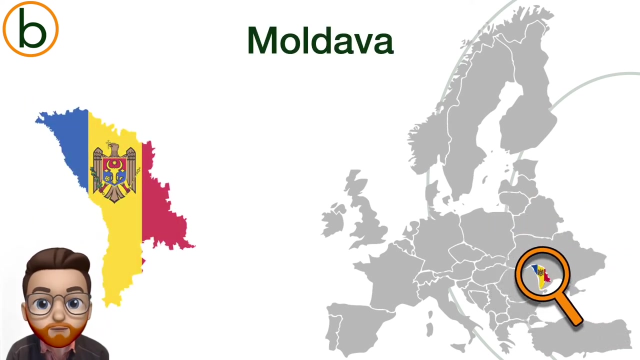 The capital of Poland is Warsaw. And then we go to the Baltic states, with Estonia That has Tallinn, Latvia with capital Riga, And Lithuania with capital Vilnius. That brings us to Belarus with Minsk, Ukraine with capital Kyiv, And Moldova with Kosovo With capital Chisinau. 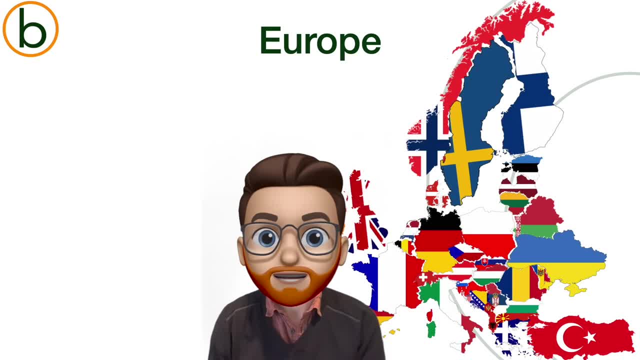 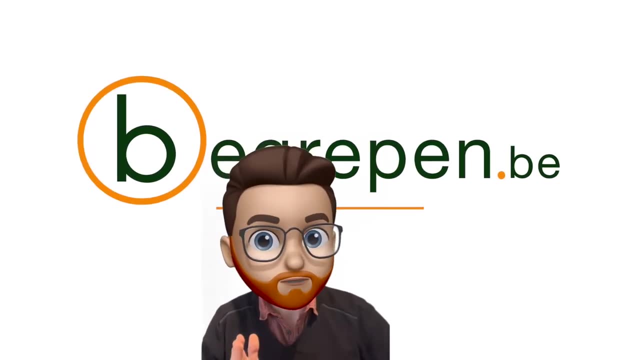 Those are the European capitals. As you can see, a lot of big countries, small countries, Countries you might have heard a lot about And countries which were quite new to you before this video. I hope you found this interesting. Stay tuned for other videos. Have a look on the channel. 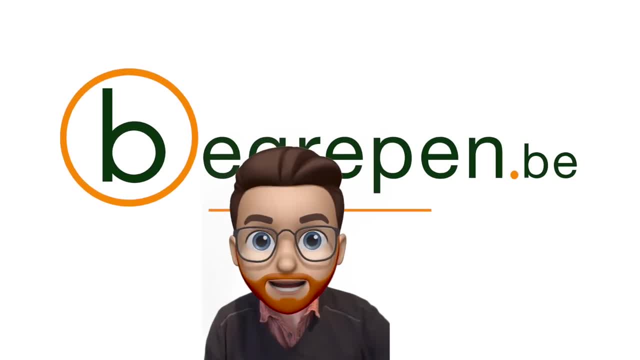 And if you liked this video, Please hit the like button and subscribe. See you next time for another Dope video. See you next time for another Dope video.